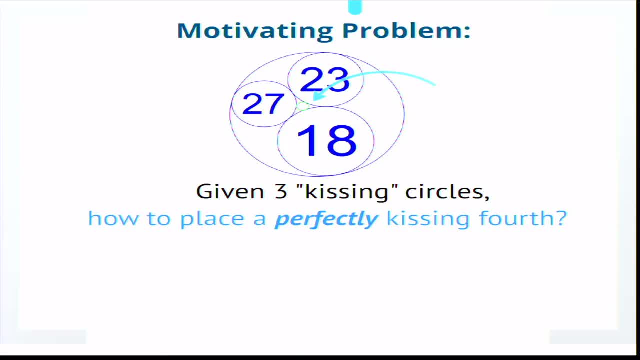 it's a vague question at the moment, how would you place a perfectly kissing fourth Okay? So this is kind of an abstract question And I'm going to start with the first one. So it's a vague question And when you kind of start digging deeper and deeper into this question, 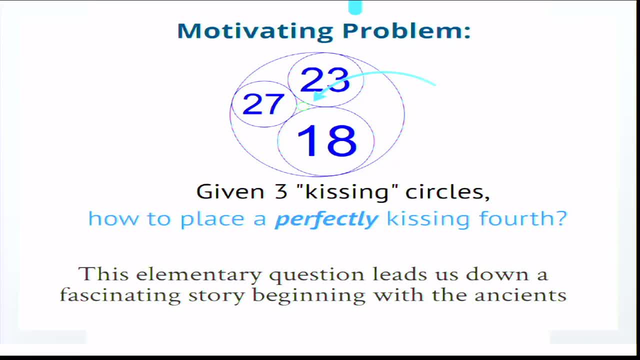 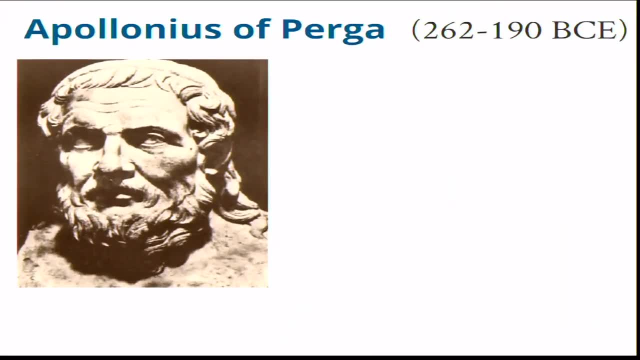 there's a beautiful story, And that's what I want to tell you. At least, I find it beautiful. Okay, So it begins with the ancients. So let's go back about 2200 years. So this gentleman has anybody heard of this guy? I'm sure this is exactly what he looks like, according to. 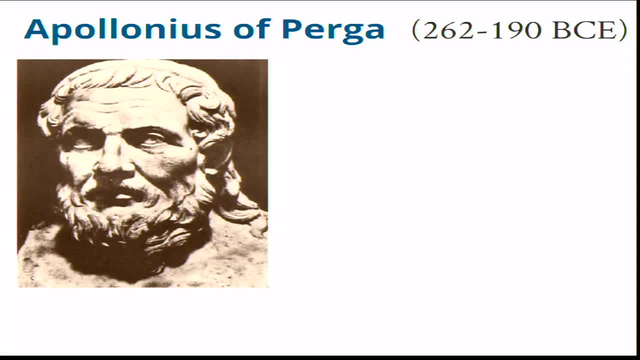 Wikipedia: Apollonius of Perga. Anybody heard of Apollonius, At least in that, Okay, Okay, So he's for us. he's kind of a famous guy. He's most famous probably. 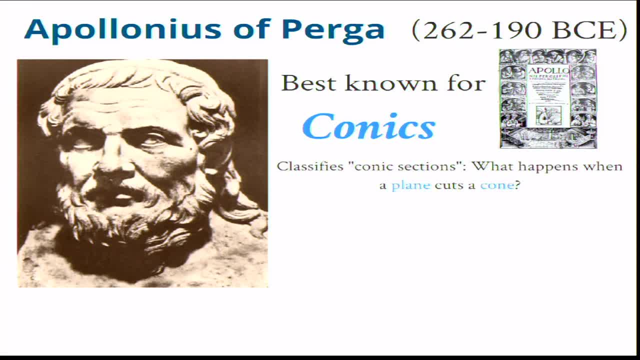 for beautiful text on conic sections. So what's a conic section? You take a cone. Probably everybody knows this And even if you don't, now you do. You take a cone, you slice it by a plane. What's the intersection? So if you slice it exactly across, you get a circle. If you slice 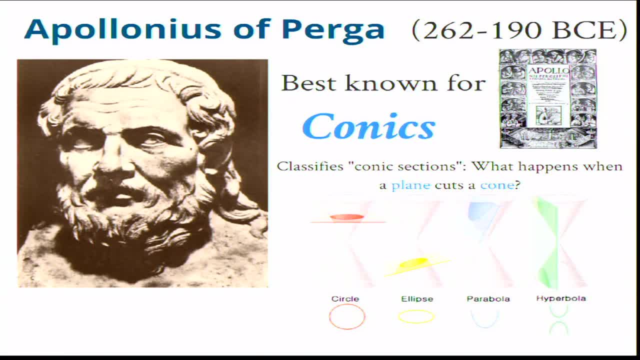 on an angle, you get an oval, clearly. But what kind of oval? You get exactly an ellipse right The focal point. Let me not define an ellipse. If you slice a little bit more sharply, you get a parabola. 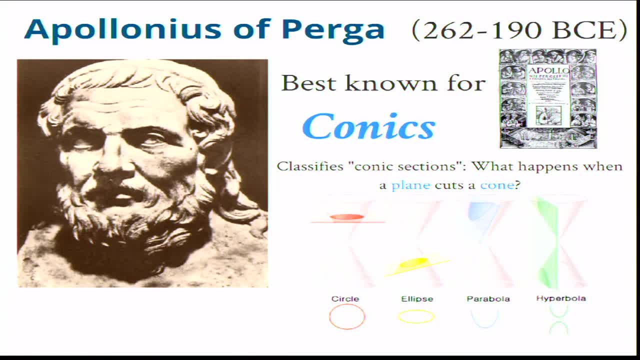 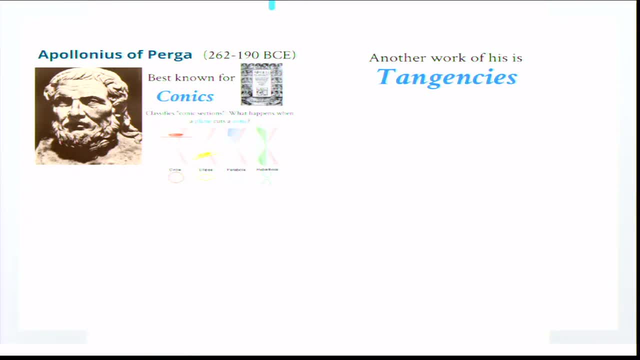 At exactly the right slope and slightly more, you get a hyperbola. In fact he coined these terms, parabola and hyperbola. So this is his kind of best known work. But another excellent work of his is tangencies, where he solves the general problem of constructing circles tangent through. 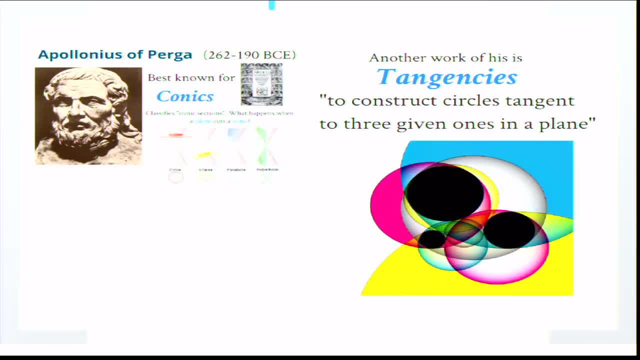 to three given ones in a plane. So the black circles have been given to you and your task is to construct a circle that exactly kisses all three, Exactly as our initial problem. And he solves this problem. And what does construct mean? I mean, obviously I could just doodle something. No, we mean in the sense of 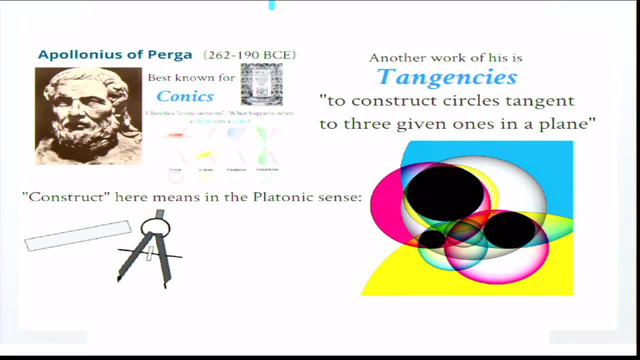 Plato in the sense of the ideal objects that for them exist in heaven, namely straight edge and compass. So he does this construction, So this solves our problem and we're kind of done, But we're not, because this book Tangencies, so conics, does survive. We have what we think is some version of conics, But tangencies we only have secondary. 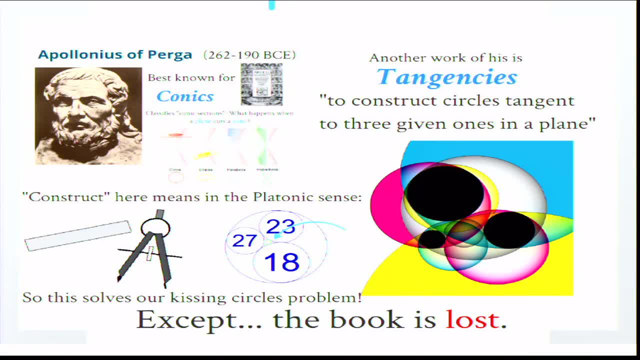 We have what we think is some version of conics, but tangencies- we only have secondary. But tangencies- we only have secondary, But tangencies, we only have secondary sources. So we know he did this, at least he has claimed to have done this, but we don't know how. 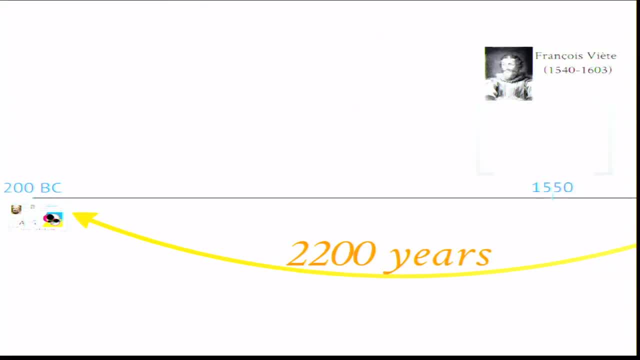 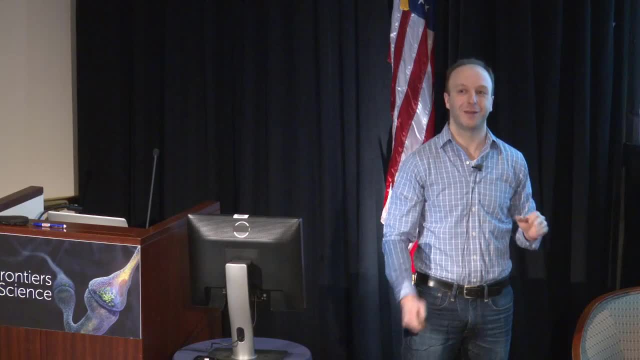 And in fact for the next 1700 years. we still don't know how. And for the last, 300 of those people are actually working on figuring out how to do it and they think maybe it's as hard as squaring the circle, and it's just he made a mistake. 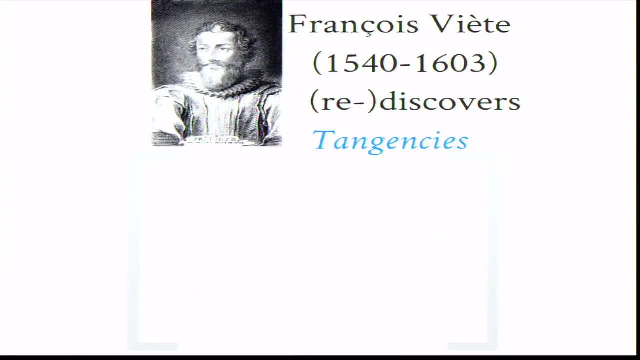 or something. It's an impossible problem. So eventually it was settled by Francois Viette in the 1500s and he has a beautiful solution which we're going to. I'm sorry, you're going to prove a theorem today. 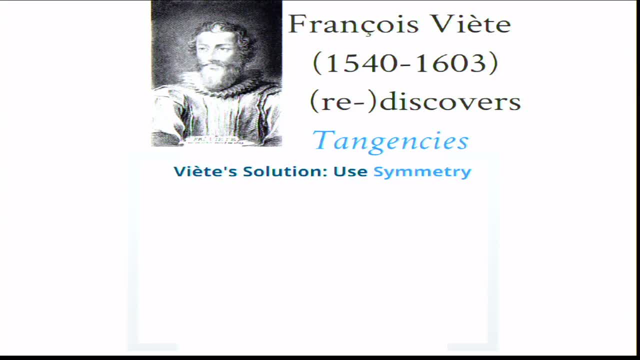 Maybe for some of you, this is a fiber that's telling you you're in box B, You're in box A, it's going to be okay, So I hope it's not bringing back some painful memories. but okay, Let's see how he did this, because I think this is just really beautiful. 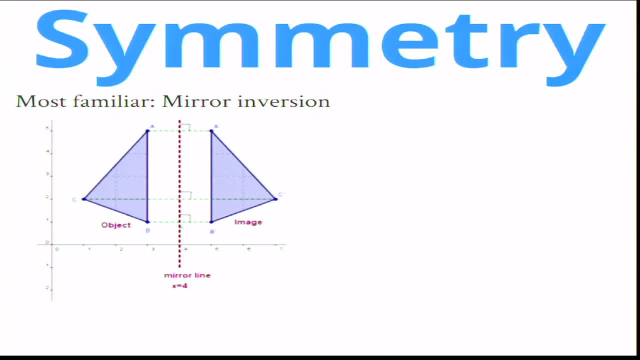 So the idea is to use symmetry, So symmetry. you woke up this morning, you looked in the mirror. you saw the mirror image of yourself. You're very familiar. A slightly less familiar symmetry in everyday life is circle inversion. So what is circle inversion? 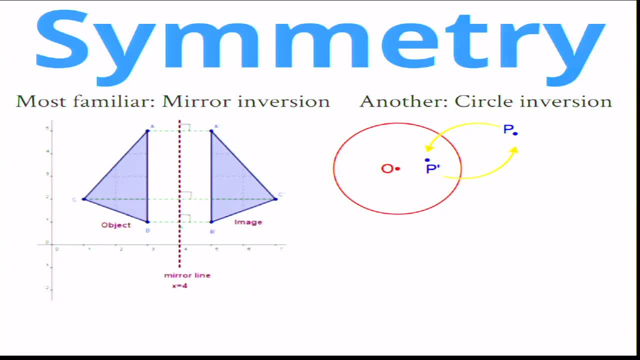 If I have a point that's ten radii away from the center, then when I invert it appears one tenth of a radius away. That's all that means. Is that clear? No, Okay, This is a point, that's so. the radius, let's say, is one. 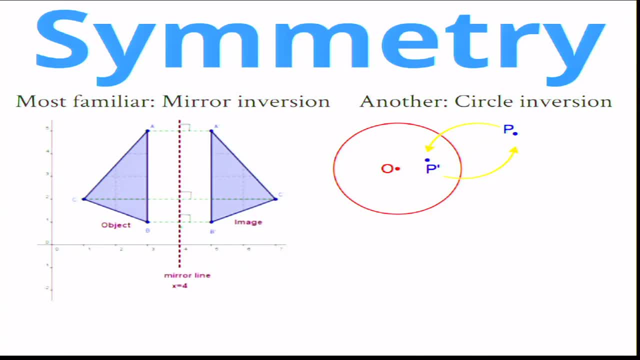 So this is a point that's distance two away from the origin. So what does it mean to invert? I just move it to a point on the same line That's half of the radius away. Now does it make sense? Okay, So if you do this? so, in other words, you want the equation, you want to be satisfied. 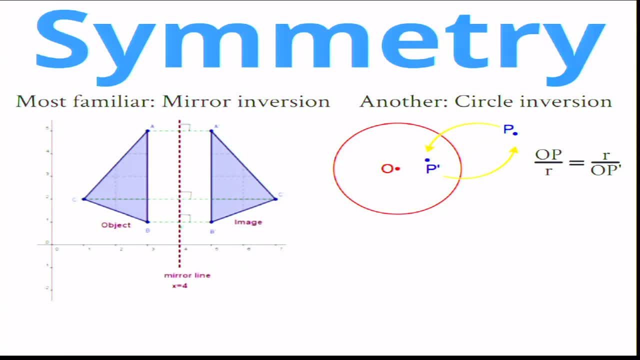 is the distance from O to P relative to the radius? is the inverse of the distance from O to P prime relative to the radius? So far, so good. Tell me. if not, because it'll make the rest more complicated, All right, So, for example. so this is Vermeer's The Astronomer. 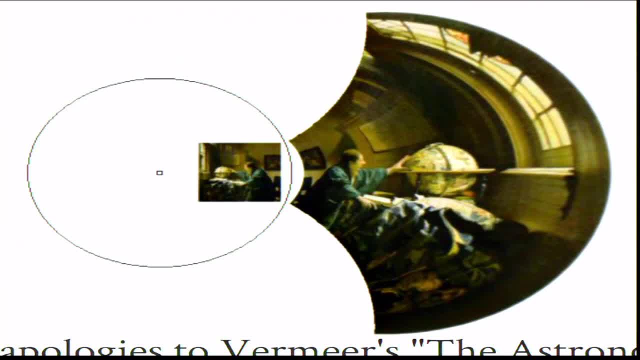 So this is Vermeer's The Astronomer, Okay, Okay. So if you take every pixel and you apply this operation by inversion through this circle, this is the image you'll get as a result. Okay, It's clear what has been done to this image. 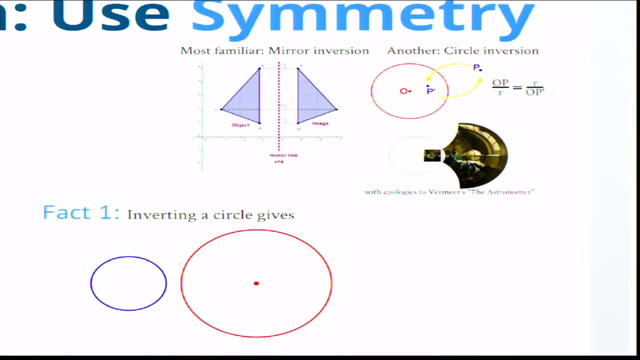 All right. So here are some facts you need to know about circle inversion, And I won't prove them, but these were very well known to the ancient Greeks. Maybe in Israel this is actually taught in the American schools. It's not, unfortunately. 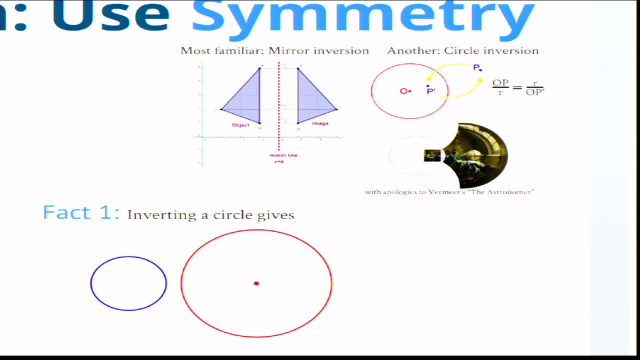 But okay, That's another topic. So if the points that you're, If the pixels that you're going to invert, are themselves already in the formation of a circle, what do you think you get when you invert this through the red circle? Does anybody not in the front row know the answer? 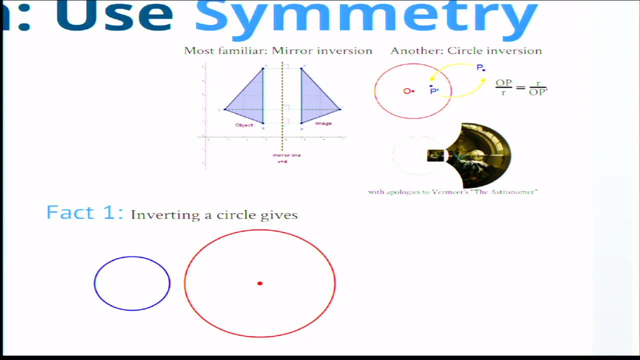 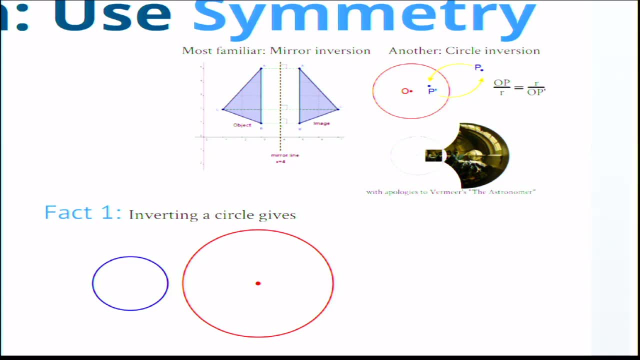 Yes. So what I'm going to do is just like we took the astronomer and inverted every single pixel by pixel. I'm going to take, pixel by pixel, these blue points and invert them through the red circle, But the points themselves are already in a circle. 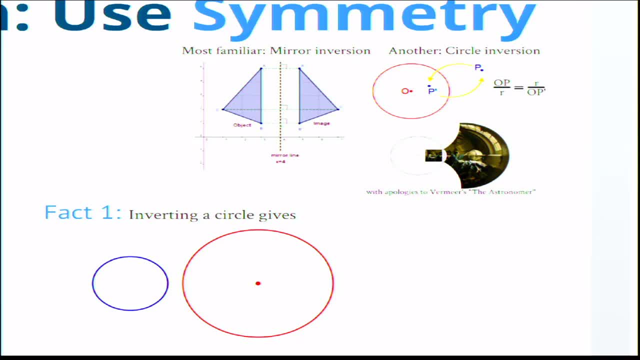 So what will we get when we do this inversion? Okay, So we can guess or we can just do it. You'll get a circle. This is not too surprising. once you've done it, It's pretty beautiful the first time you see it. 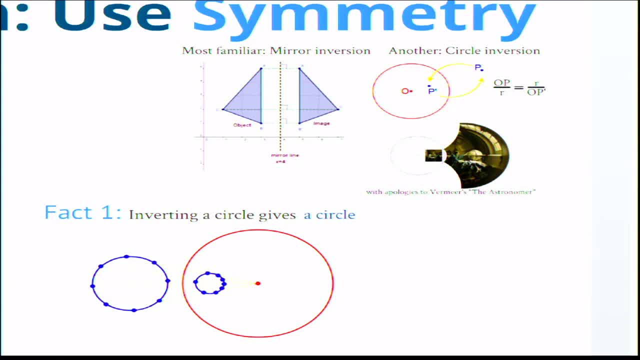 But there's been some squishing of the. So these are equally spaced points and I've moved them individually And you see they squish some places and stretch some places. So it's still in totality a circle, but there's still some squishing. 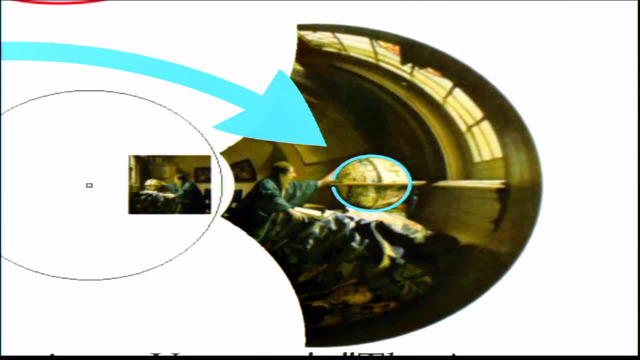 And actually we should have seen that already, because the astronomer's globe remains a circle. Okay, So that's fact one. Fact two is what happens if you invert a line. So if the points you had, these blue points, are aligned, I'm going to invert them through. 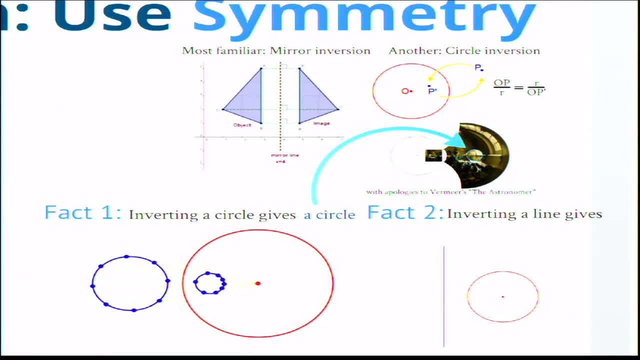 the red circle. Now, what do you think is going to happen? You'll get a circle again, And because the line gets infinitely far away from the center of the circle, the circle that you get, the reflection, will be infinitely close to the center. 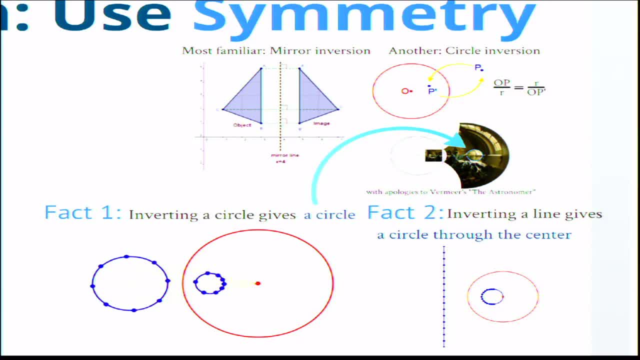 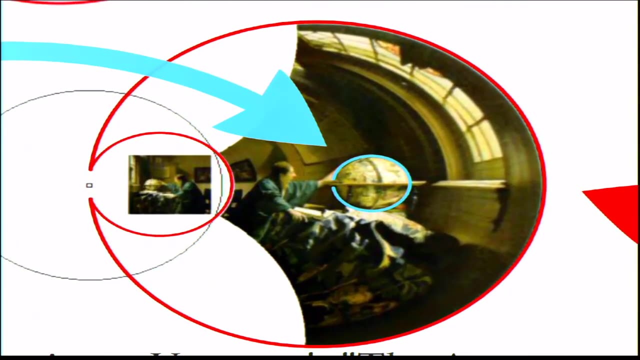 And you get a red circle that's in the middle of the circle. the reflection will be infinitely close to the center, So you'll get a circle again. In other words, it will pass through the center. Does everybody see that? And again, we should have seen that in the astronomer, because if you look at this edge, 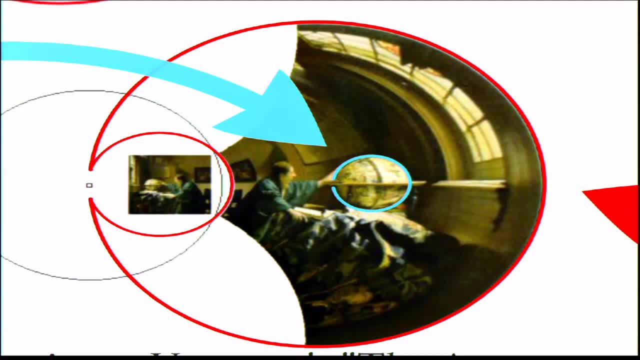 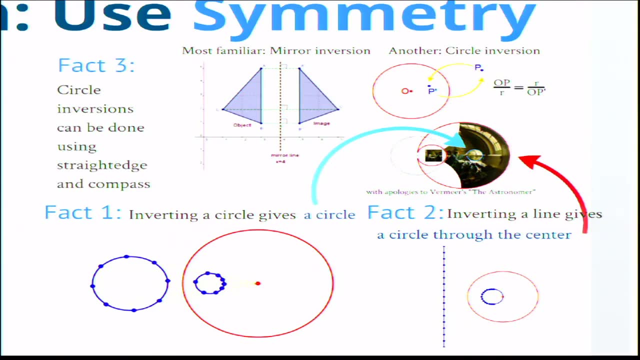 the edge of the astronomer is a line, or at least a line segment, and the inversion of that is this outer segment which, if we continue the arc, goes to the center. So far, so good. So, armed with these two facts and another fact, which is that these operations can be, 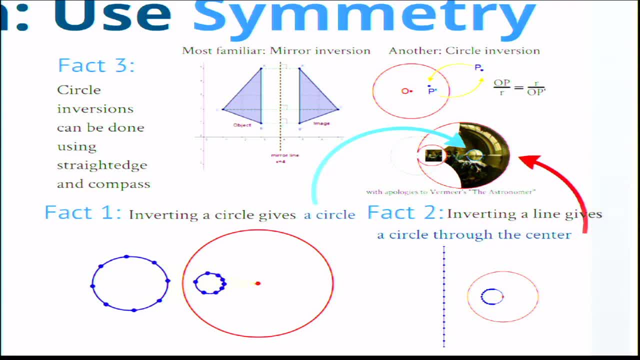 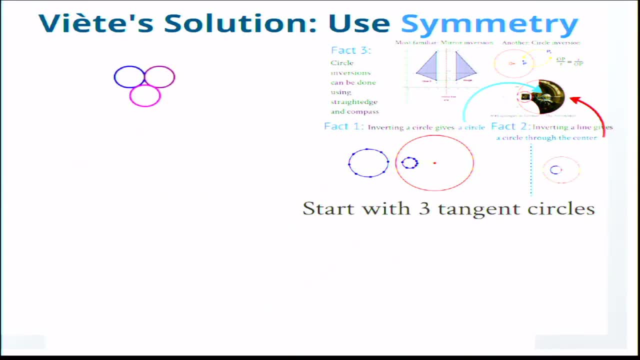 done by straight edge and compass. and maybe fact four is that all of this was very well known to the ancient Greeks. we can see Viet's solution. So you start with your three tangent circles, just as we did in the very beginning, and 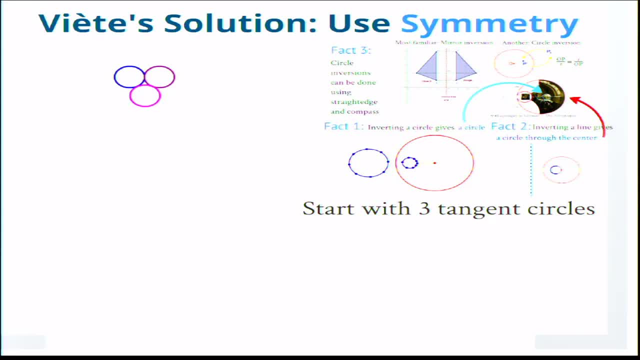 now what So? you go for a walk in the woods, you get a coffee, you check your email. you're still stuck and you sort of stare at this thing and go. I don't know what to do. And that's what happened for 300 years. 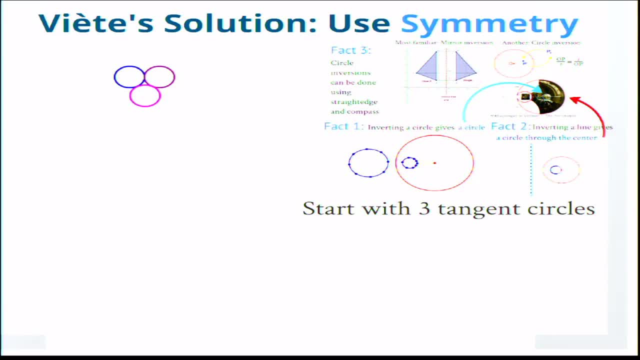 Okay, Until Viet said: here's an idea, and it's a totally wild kind of out of the blue idea. Let's put a point at one of the points where two of the circles meet, and I'm going to draw an auxiliary, a completely arbitrary circle that's centered at that point. 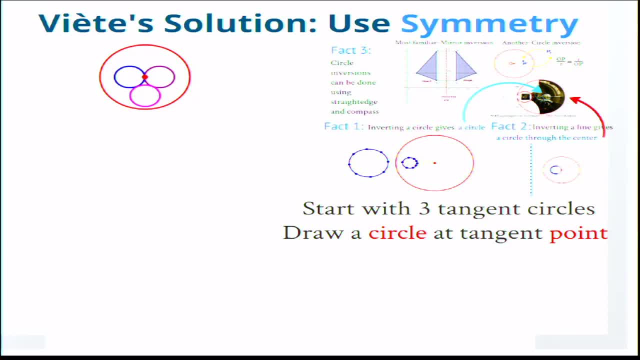 I hope your spidey sense is starting to go off. Something's about to happen, Okay, Why would I have done that? Well, what am I going to do with that circle? I'm going to use that circle to, Okay. 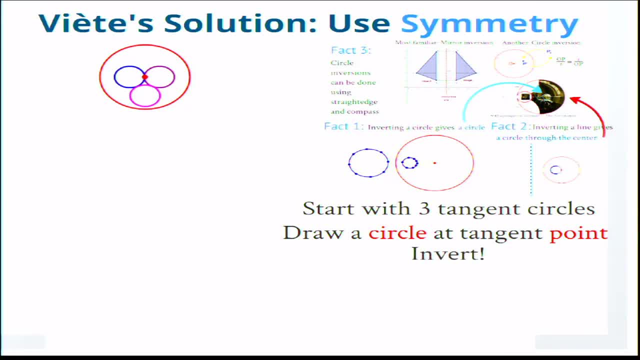 Invert the entire configuration. So what happens if I invert this blue circle through the red circle? So the red circle is my mirror. I invert the blue circle, I get a line, because it's a circle through the origin. Okay, You guys are very good. 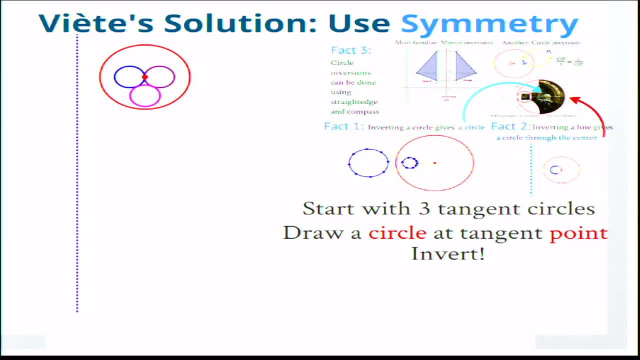 I get a line because it's a circle through the origin. What happens to this purple guy? A line and this pink guy is a circle. so this is the configuration you get when you do the inversion. But now the solution is completely trivial. 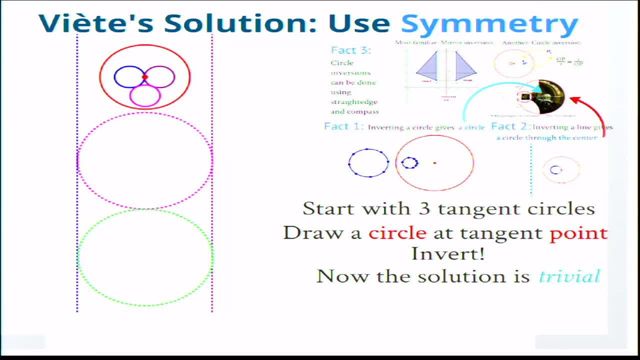 I don't think I have to convince anybody that you can draw this circle with straight edge and compass Now what Invert back? Invert back, Exactly Okay. Quitterat demonstratum. I hope you survived that one, Okay. 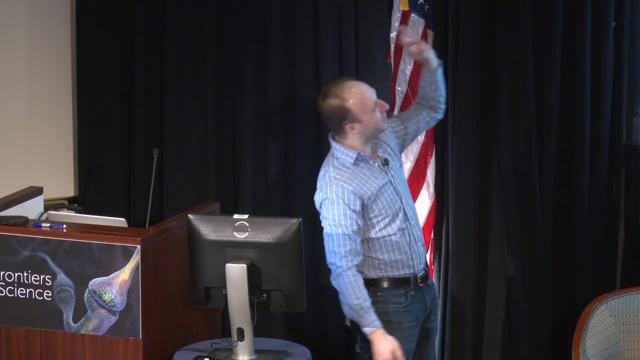 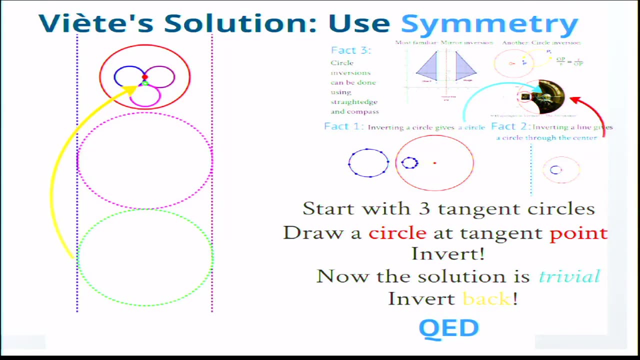 But you can see that once it's a three-line proof, once you have this stroke of genius to put a point at the tangency and invert- And that sometimes takes 300.. Okay, So now we kind of have a solution, Okay. 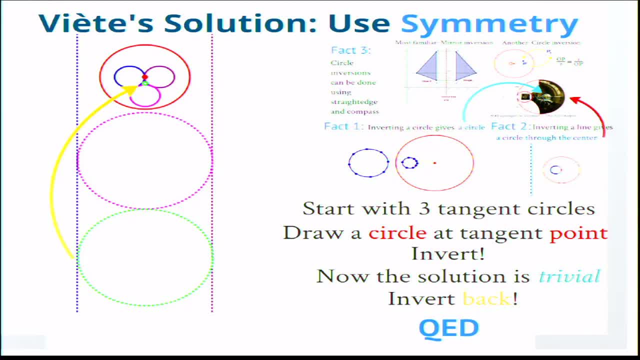 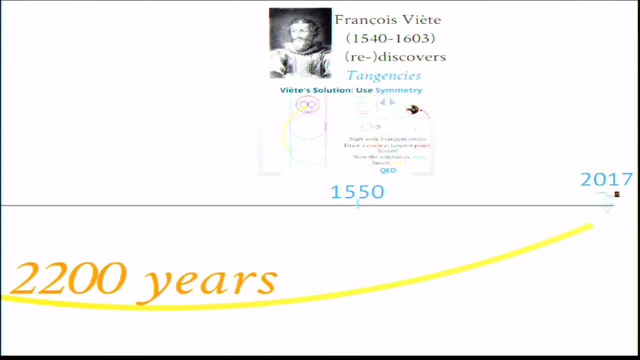 So we have a solution to our original problem if we're satisfied with the fact that, yes, we can do this with, you know, heavenly, straight edge and compass. But actually there's more to the story. So, another 100 years later, this guy, Rene Descartes, starts doing redoing all the geometry. 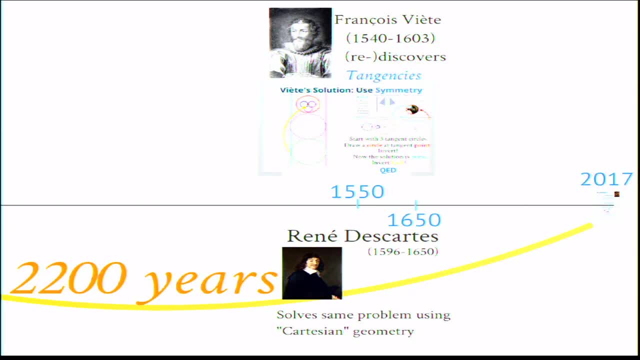 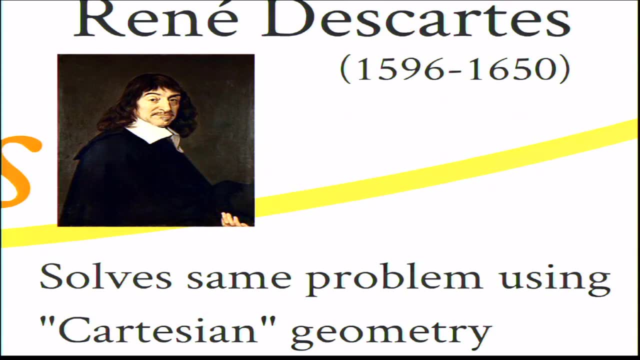 that we know in coordinates, because he discovers Cartesian right. he discovers coordinates. So if you're the guy that invents the thing, you go back and look over everything and he discovers a beautiful relation. So when there are four circles that are mutually tangent and their radii are R1, R2, R3, and 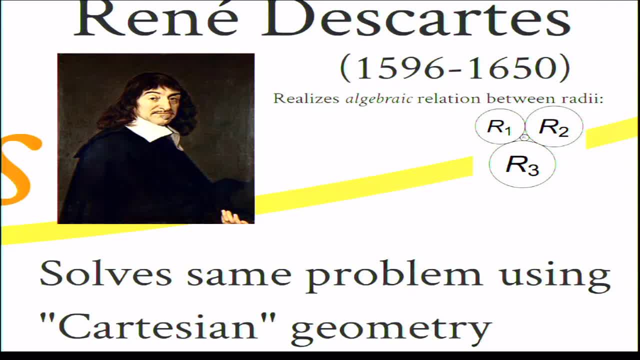 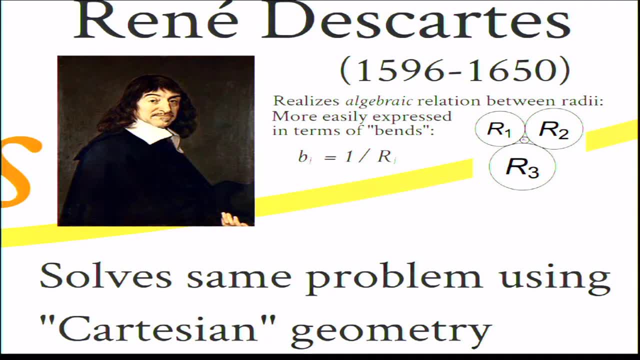 R4, then there's an algebraic relation between them which is more easily expressed in terms of what one may call bends. So the bend of a circle is the reciprocal of the radius 1 over the radius. So in our example, actually, that's what these numbers were. 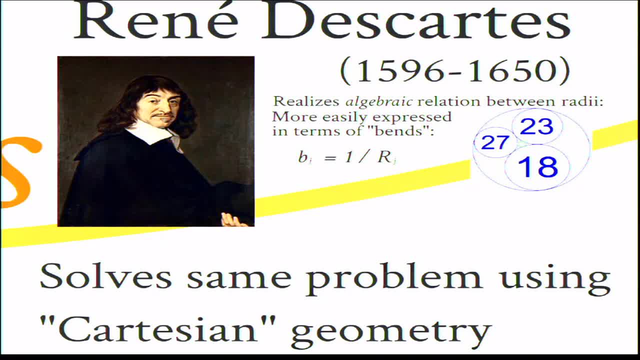 So this is a circle of radius 1- 18th. This is a circle of radius 1 over 23,, 1 over 27.. And the relationship is: there's some if you take the squares and sum them, or if you. 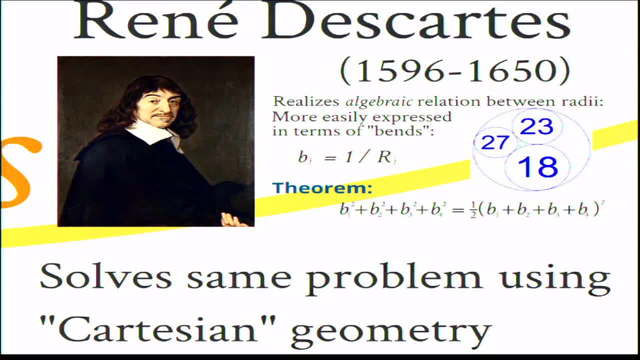 sum the bends and then square, you'll almost get the same thing. You'll be off by a factor of a half. OK, I'm not going to prove that theorem for you, But that's again. this is everything that I'm saying today, that I actually well everything. 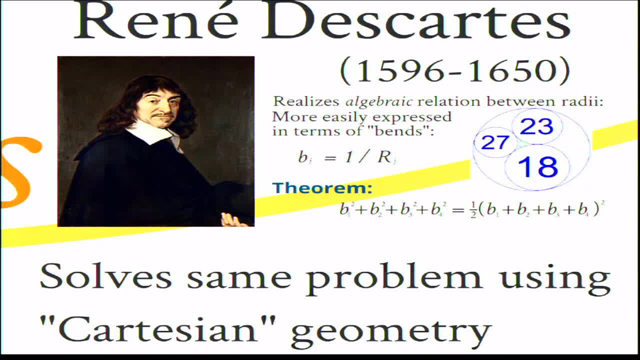 that I, that I that you should understand is: you know this is a high school level theorem, This, if we had a half hour I would prove it for you. I'm not going to, And you know so. 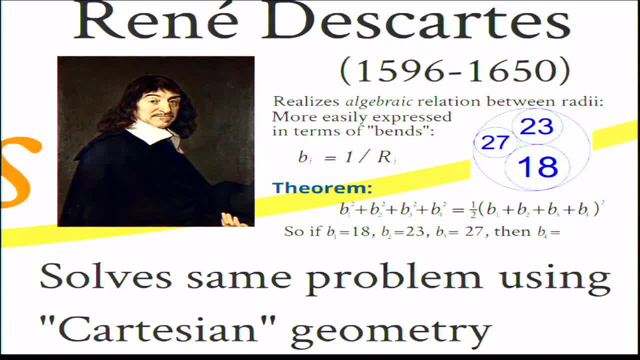 OK, And well, what does that mean? Well, that means that if we, if we're given these initial three- 18,, 23, and 27,- then three of the variables are no longer variables. You have one variable: quadratic equation. 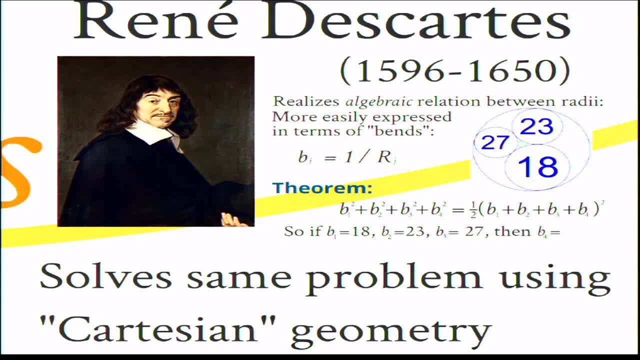 Again, this is in Israel Elementary School. OK, or something You can compute that the curvature of this inside circle, the bend of this inside circle, is 146.. In other words, not only can we put it there with straight edge and compass before we 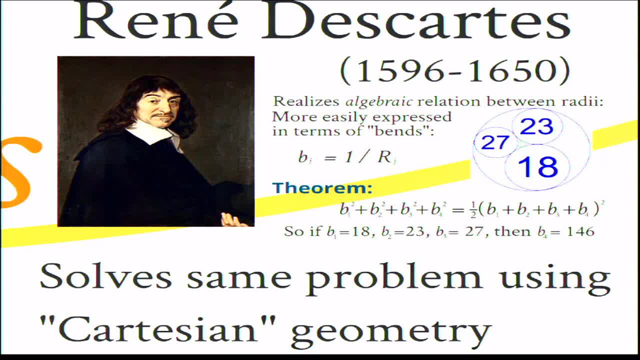 do it. We're not going to measure what we get, We'll just have a theorem that tells us what the radius is of the circle. So it's a circle of radius 1 over 146.. Is that, is that clear, OK? 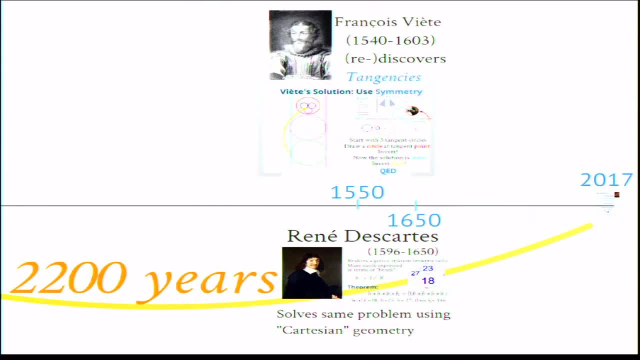 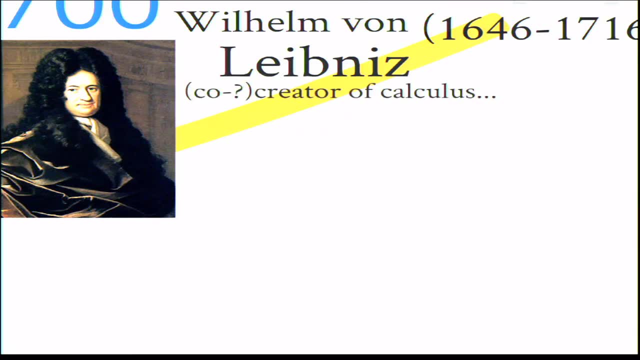 So again, we've basically answered the problem, but that's not enough for mathematicians. They keep scratching. And the next one is this guy, Leibniz, which, if you're German, he's a co-creator of calculus. 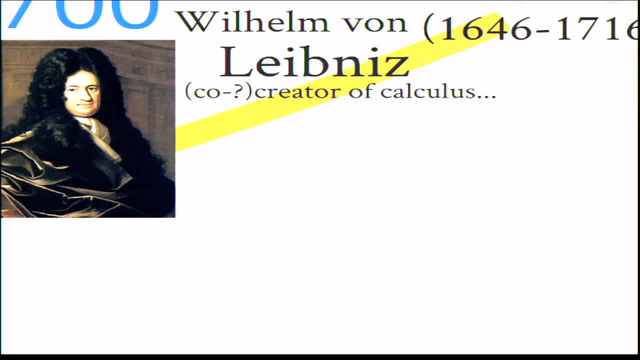 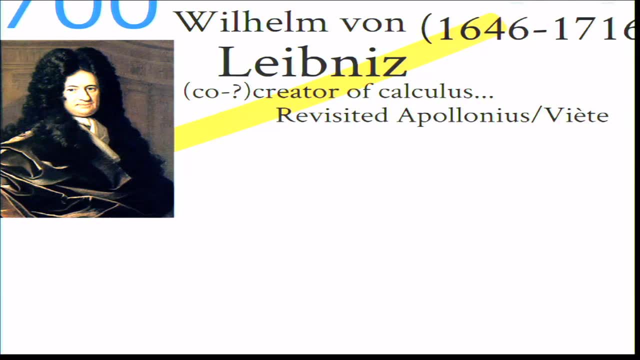 If you're British, he's a rotten scoundrel. That's a whole other topic for a whole other time. OK, But like all mathematicians and scientists before him, he revisits these questions of Apollonius and Viet and so on, and he has a very interesting insight, which is that 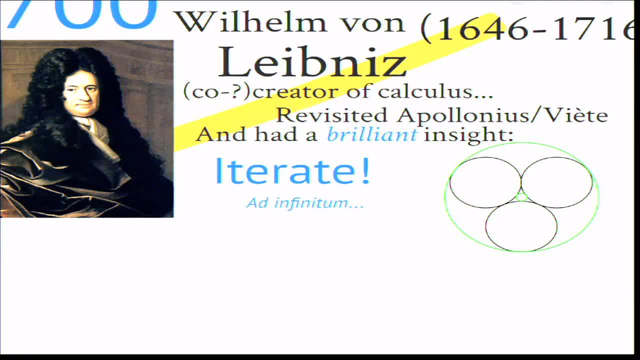 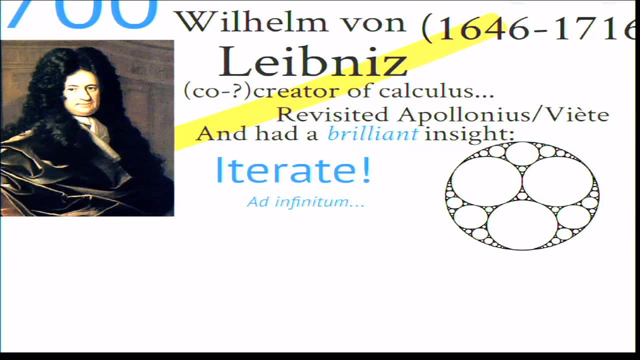 once you have done this straight edge and compass, once you can switch which three circles you have, And you can do it again, and again, and again, forever. And he's the first one to draw this beautiful fractal. Unfortunately, in the 20th century it's not his name that got attached to it. 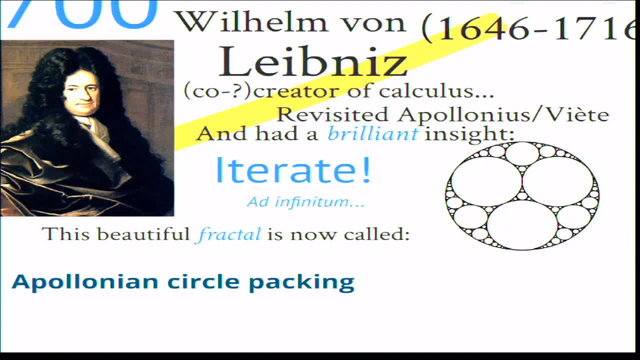 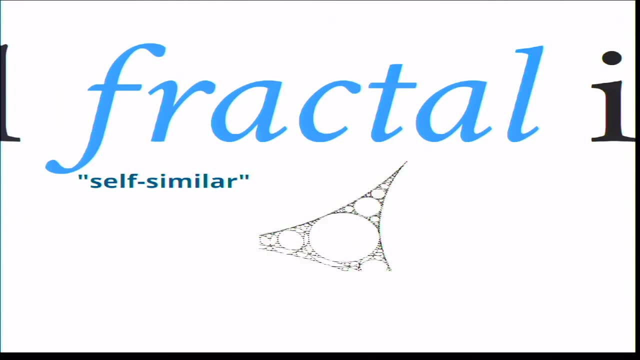 It went all the way back to Apollonius, although Apollonius never actually saw this picture. So it's called an Apollonian circle packing. What is a fractal? Let me give you a definition by example. It's something that's. I think you guys know what a fractal is anyway. 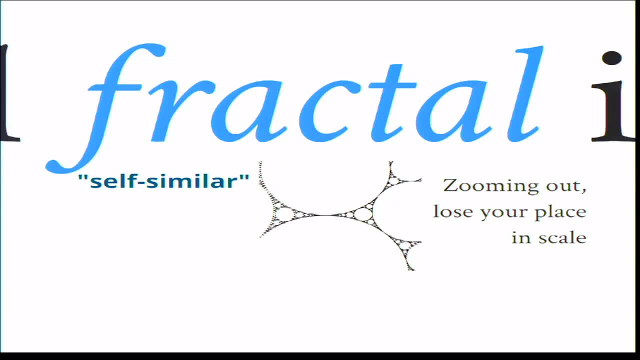 You can't tell the scale as you zoom- In this case, I'm zooming out. You can't tell if we're at the picometer, nanometer, kilometer. You don't know where you are. Everything looks the same. 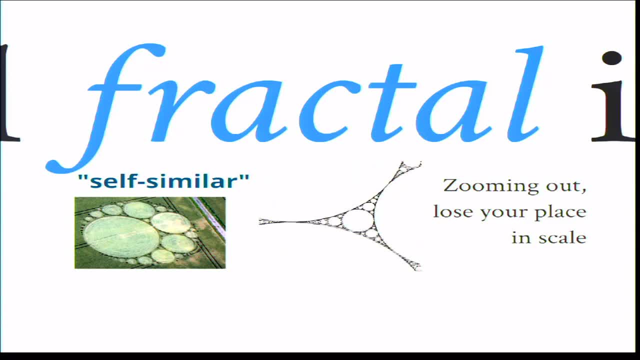 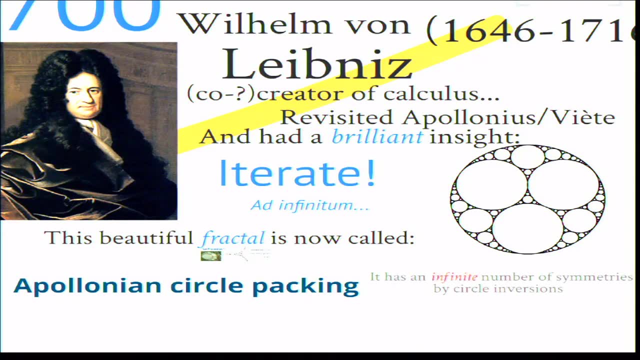 And I guess aliens like this thing. OK, I guess aliens like this thing so much they decided to build spaceships and land in England. OK, So that's the Apollonian circle packing. It has infinitely many symmetries once you construct this infinite object by circle inversion. 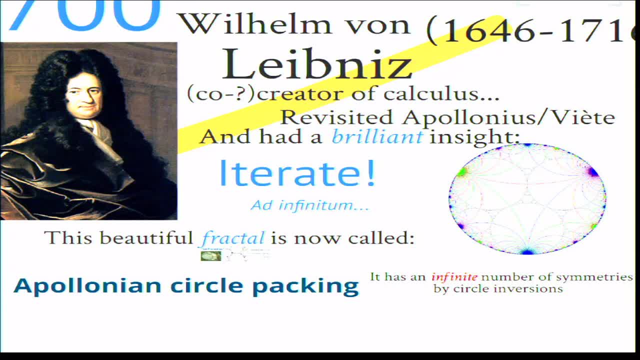 So these are some of the symmetries. I hope you see that if I take this circle and I reflect that one, I'll get that one, and so on. These symmetries arise in lots of others. OK, These are some other things that you maybe are familiar with in the arts. 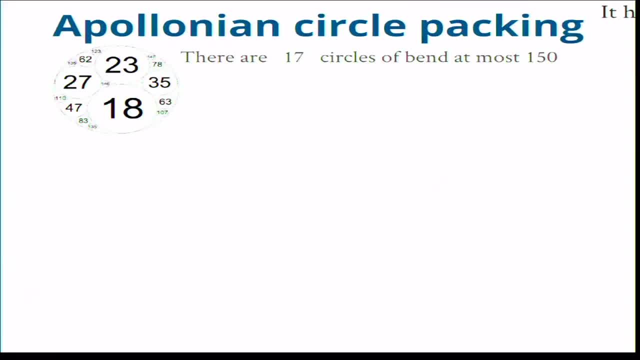 So let's ask another question about this Apollonian circle packing. So, as we do, as Leibniz is sitting there putting in more and more circles, if he restricts himself to circles of radius at least 1 over 150, right, he's not going down too deep. 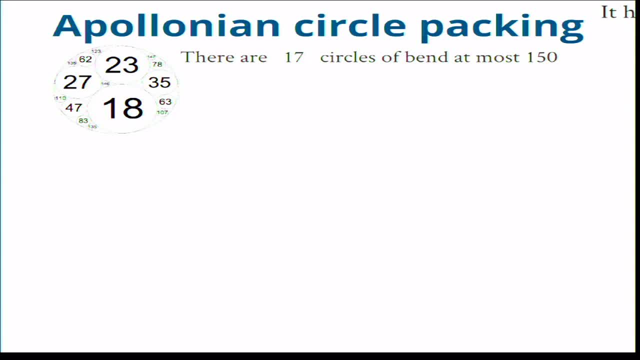 In other words, the bend is at most 150.. So these are all of them, And you can count them, and there are 17 of them, And if he spends a lot more time and goes out to 1,000 bends- at most 150, then he's. 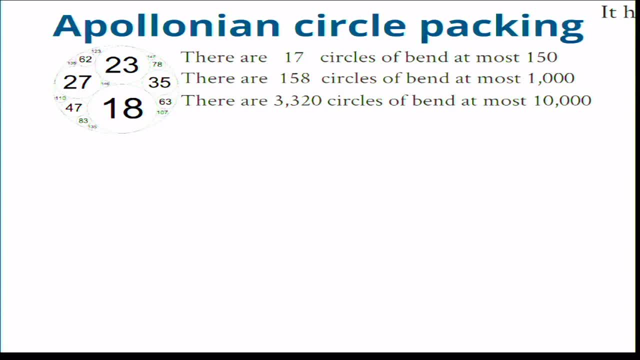 at most 1,000.. He'll be drawing 158 circles And if he now he needs a computer probably- I don't know how much time he has on his hands- So if he allows himself really really tiny circles of radius 1 over 10,000, he's going. 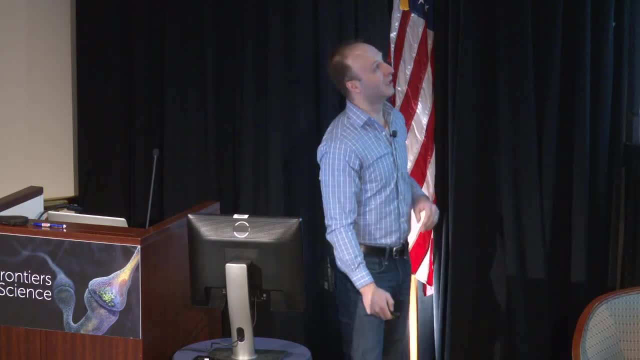 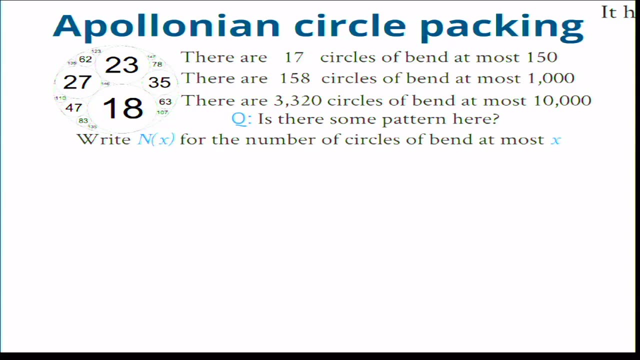 to draw 3,000 circles, And the question is: is there some pattern to these numbers? So let's set n of x. sorry, there's going to be a function warning. n of x is the number of circles of bend at most x. 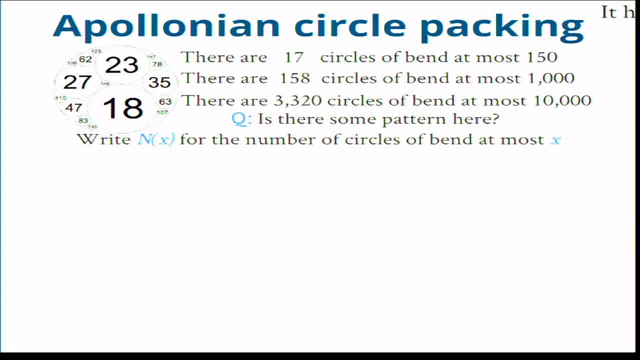 So n of 10,000 is 30.. OK, OK, And you plot this thing And you see a nice, a nice shape. And just for comparison, here's a graph of y equals x And here's a graph of y equals x squared. 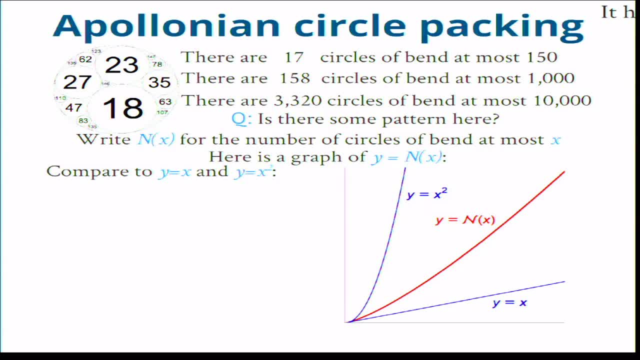 I'm obviously playing with the axis to make it visible. So what's going on? So this is a theorem from a couple of years ago with a collaborator, Yo, that says, in fact, the asymptotic growth rate is some power. 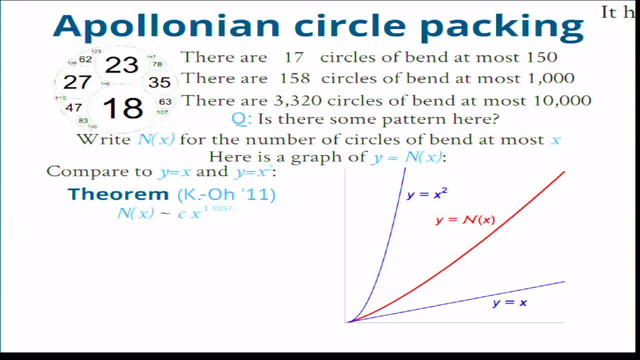 But that power is some fractal power, So it's not a. you know, the power law is 1.3, something. OK, Stare at the red line for a second. So this is the actual data. That's this side. 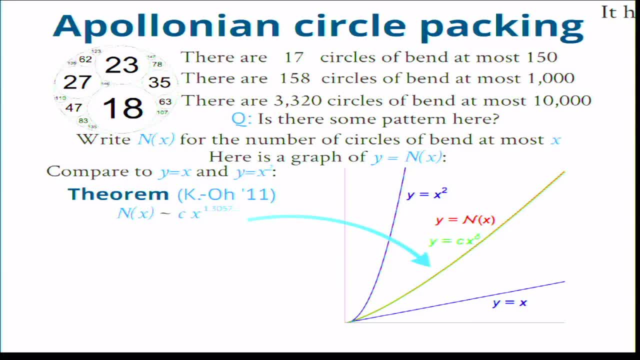 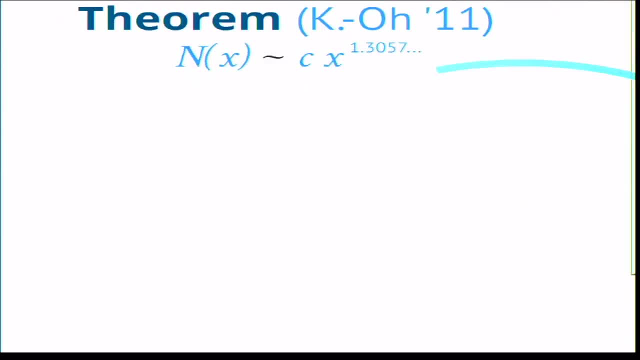 And now I'm going to plot this side, which is the predicted data. That's the green line. OK, So that's what this squiggle means. The ratio of the two goes to one. Let me give you just one hint on the proof. 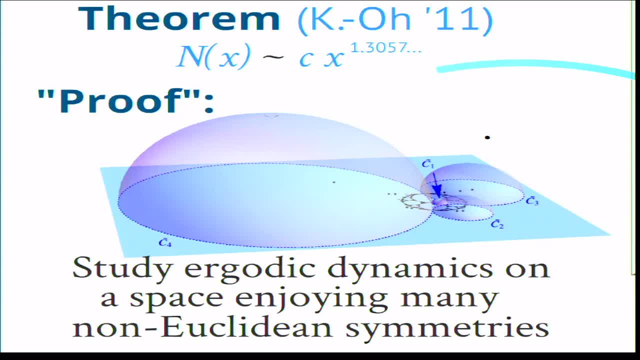 OK, I guess I'm not really going to say anything about this, except that it's an instance of the space you're looking at isn't really the space you should be looking at. So what's really happening in this picture is you have the fractal that's lying in the 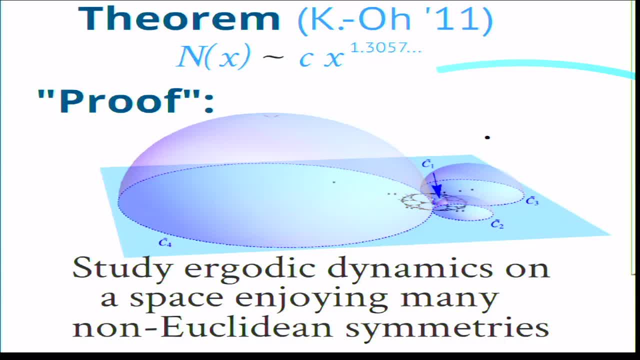 plane. But actually it's an action. What you should be thinking about is the action in hyperbolic three space. that- and you study some chaotic dynamics on this system- prove some ergodicity. It has non-Euclidean symmetry. 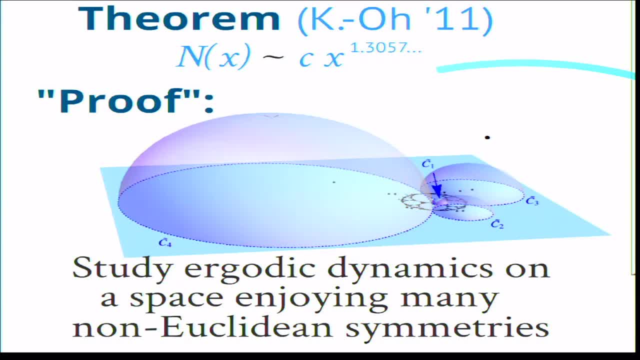 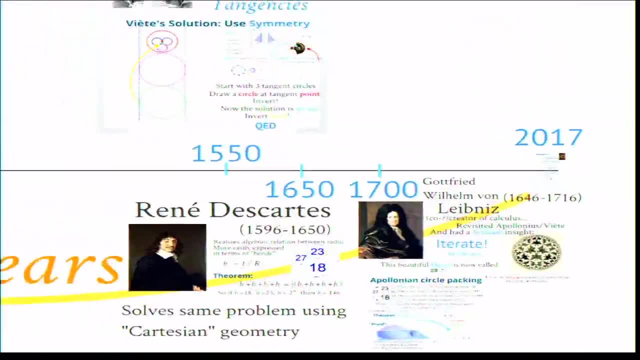 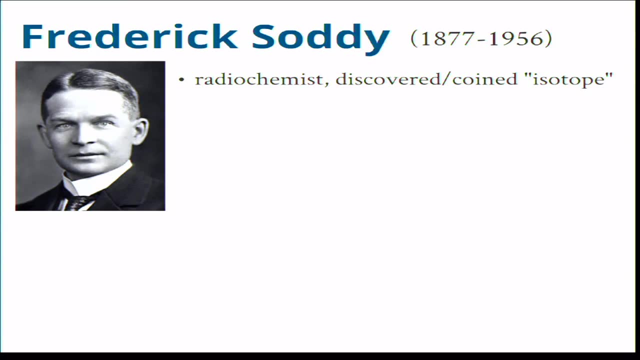 So Uri's talk will go much more into that. It will go much more into not this particular picture, but other instances of when dynamics can tell you something about other things. OK, Very quickly, let me tell you the rest of the story, which comes from, actually, a radio. 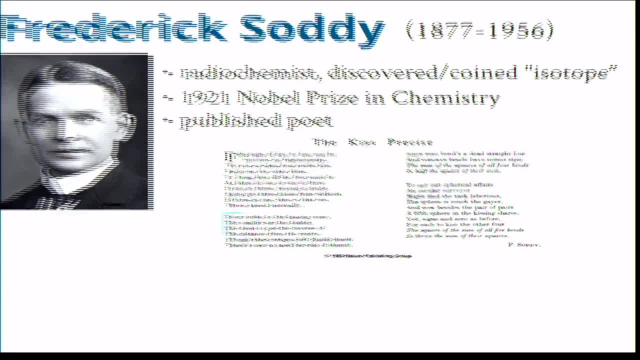 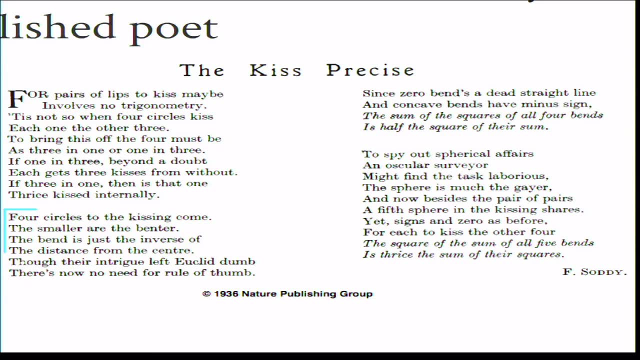 chemist, so Frederick Soddy, a Nobel laureate in chemistry and a published poet. So here's a little bit of the poem. Four circles to the kissing come. The smaller are the benter. The bend is just the inverse of the distance from the center. 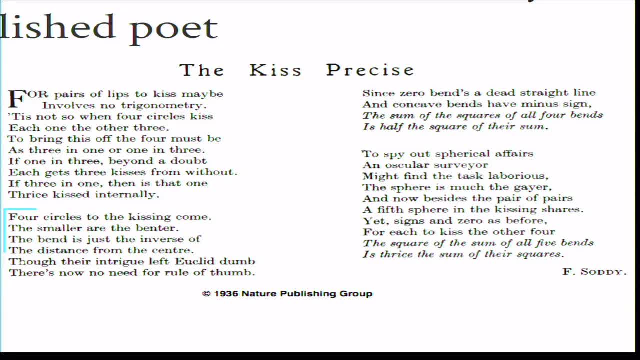 Left: Euclid dumb. there's now no need for rule of thumb, since zero bends a dead straight line. So if the radius is infinity, that's a straight line. That has bent zero, And concave bends have minus sign. The sum of the squares of all four bends is half the square of their sum. 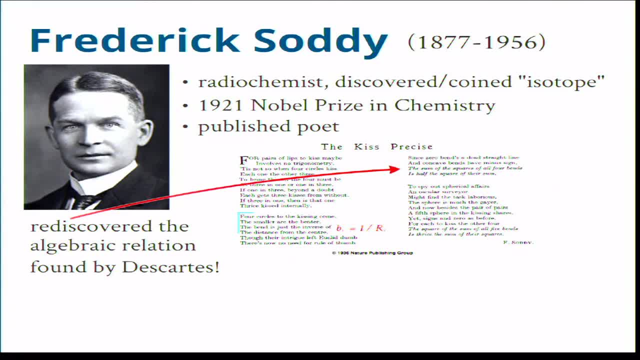 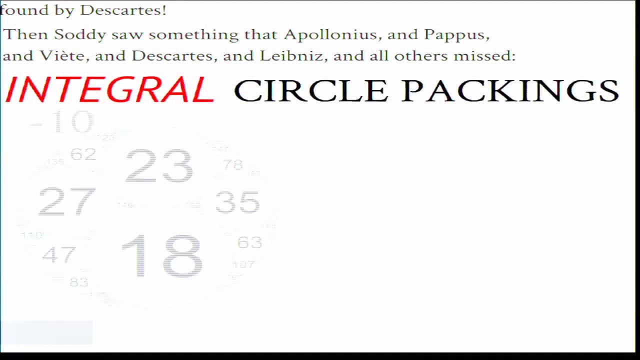 I hope that's familiar. So the bend is one over the radius. But that's exactly what. that's Descartes' relation, so he's rediscovered it. Then he saw something that everyone else had missed, which is when you do this circle packing- 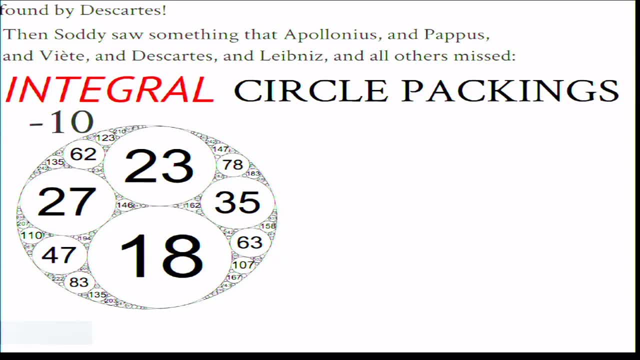 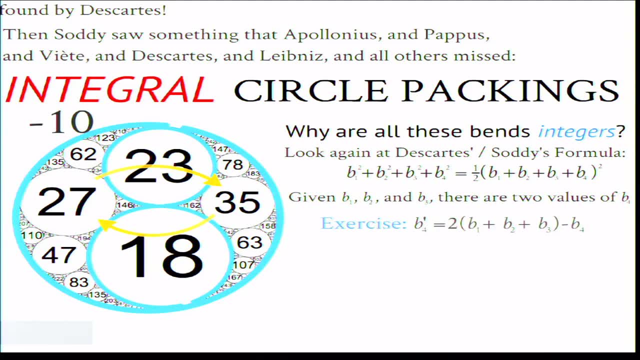 why? Because it covers integers. Where's the pi? Where's the square root of two? What's happening here? So let me not go through this in detail, but you will actually see the consequences of this kind of a relation in Charlie's talk appearing in a completely different context. 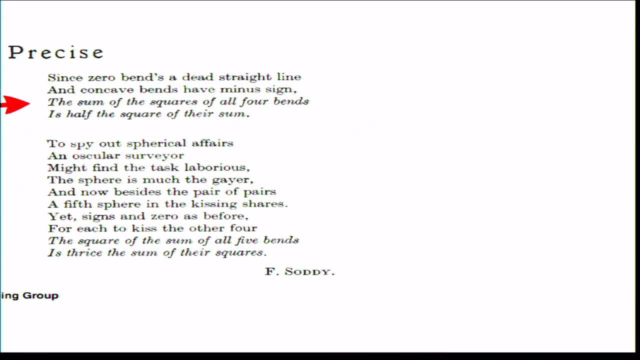 And let me just finish out the poem, To spy out spherical affairs. an oscular surveyor might find the task laborious. The sphere is much the gayer. And now, besides the pair of pairs, the fifth sphere in the kissing shares he had signed. 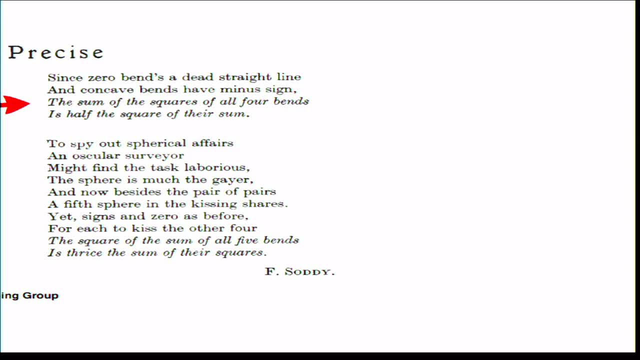 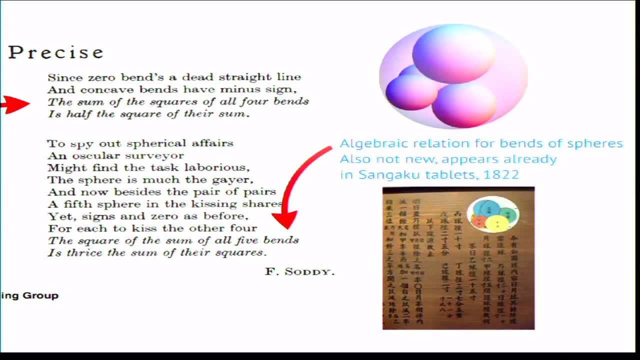 zero as before. for each to kiss the other four, The square of the sum of all five bends is thrice the sum of their squares. So this is something about sphere packings. And again he's discovered some algebraic relation. Now he's only 100 years old. 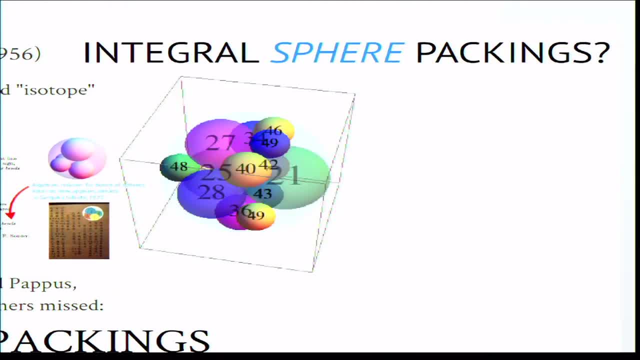 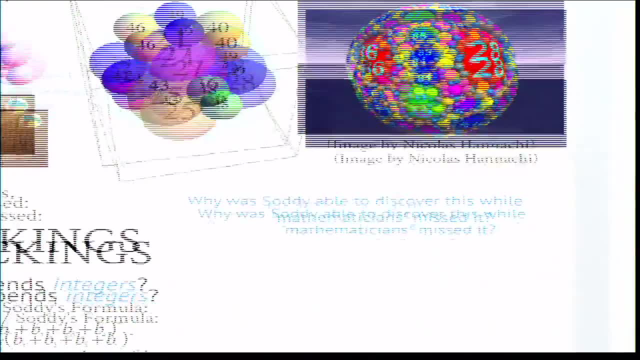 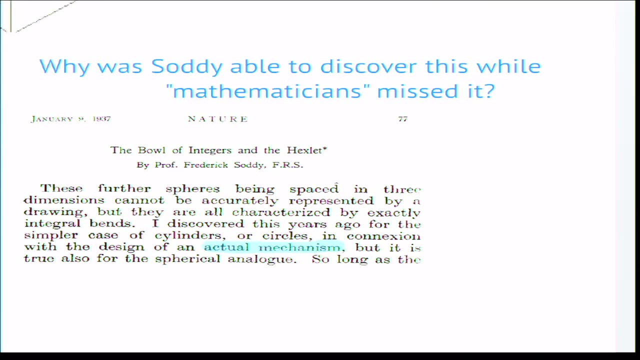 The Japanese knew this, And that leads to integral sphere packings. and here's an example of that, Just for one second, Just kind of philosophically. how can mathematicians miss this fact? And it took a chemist to figure it out.